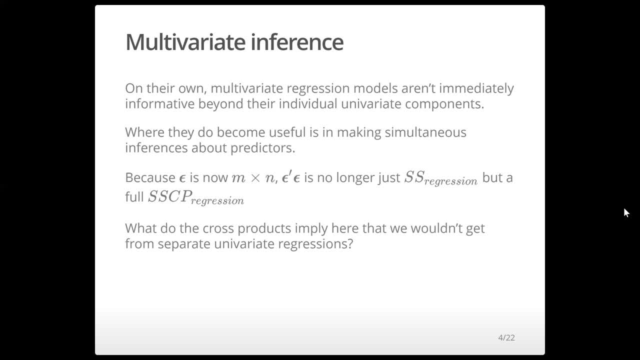 ahead and do some imprints and then we're going to roll it across the table. So that's the first thing that you have to do, is you're going to find out that our individual univariate counterparts have been relatively informative as their individual univariate counterparts—or their components. So where they do have some utility is in making 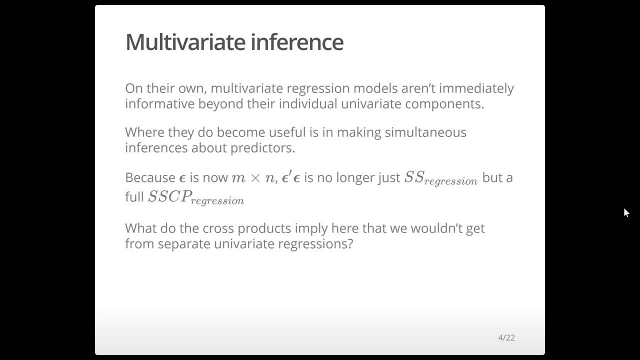 simultaneous imprints about predictors on multiple response variables. So because our residuals are now m by n. so when we do e transpose e, this is no longer just the sums of squares but it's a full sums of squares and cross products. And so what does this imply? 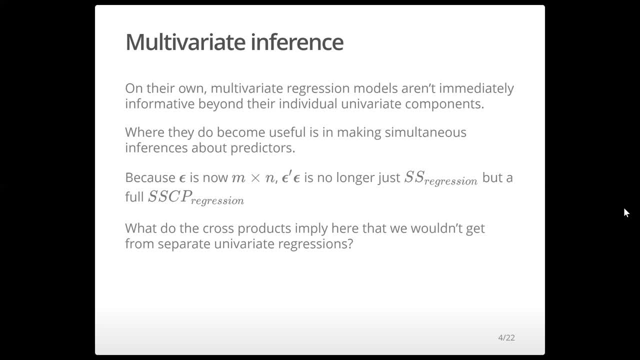 What does having cross products for our residuals imply? that is different from the separate univariate regressions. So it implies that the residuals might be correlated across the different response variables. So this is the extra information that we can test is whether the predictor variables also predict the correlation in the residuals. 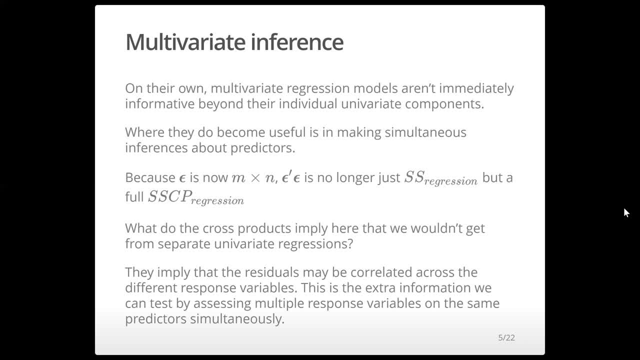 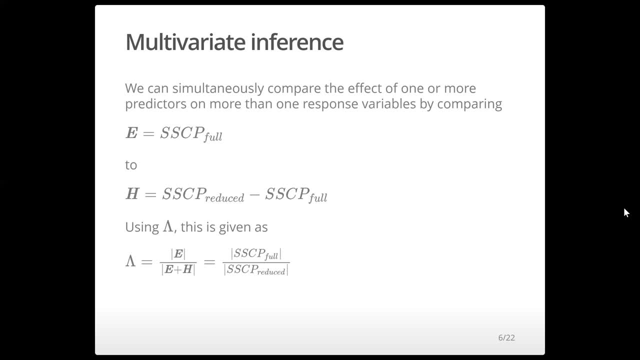 or the correlation in the response variables. So we can simultaneously compare the effect of one or more predictors on more than one response variables by comparing the E matrix, which is just the SSCP from the full model, to the H matrix, which is the SSCP reduced model. 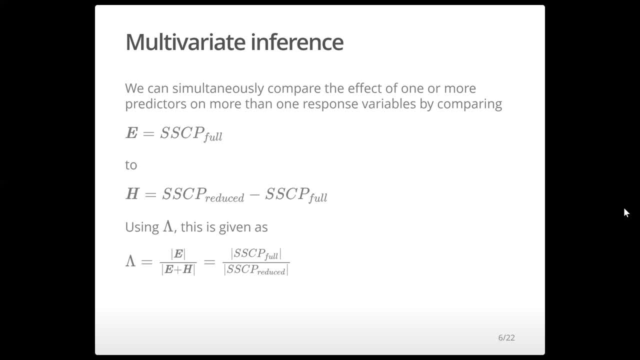 minus the SSCP full model. So it's the difference, the change in in sums of squares, it's how much of the sums of squares are reduced in the full model of the sums of squares and cross products. And so using the lambda statistic, we can test this. 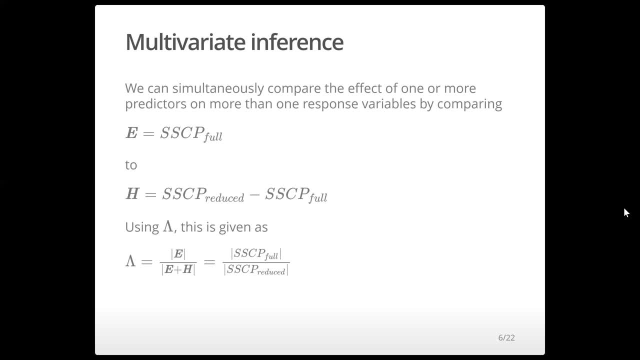 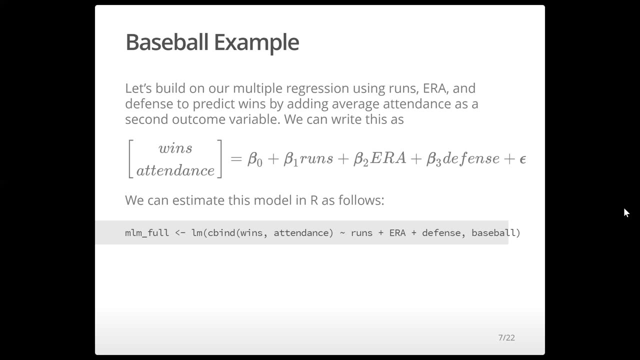 as a determinant of E divided by the determinant of E plus H or the sums of squares cross products. full divided by the sums of squares cross products will be the determinant. So, building on our multiple regression using RUNZ-ERA and In LEDS defense to predict, to predict predict wins, we simply add the second response variable in here. 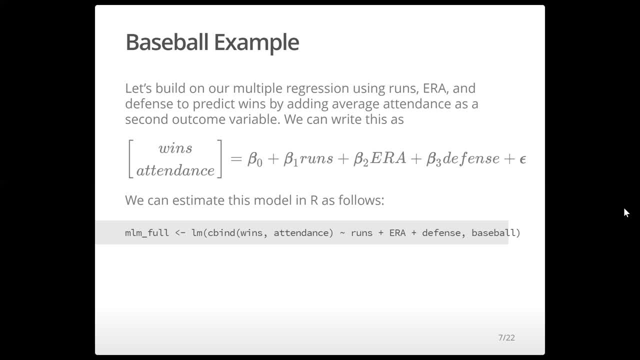 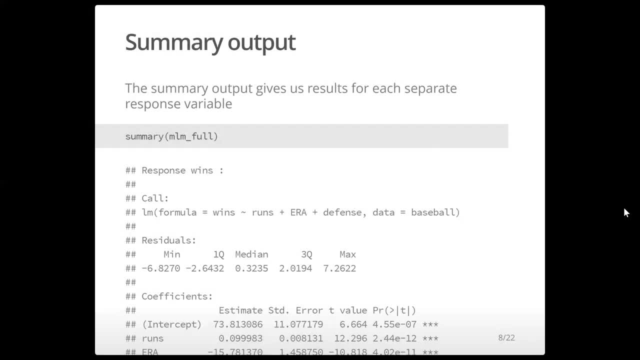 and so we can estimate from the model, as we've seen, just by c, binding the response variables and then having our predictors on the right hand side, just like in a standard regression equation, and it gives us the summary output for this mlm object, is going to actually give us just two. 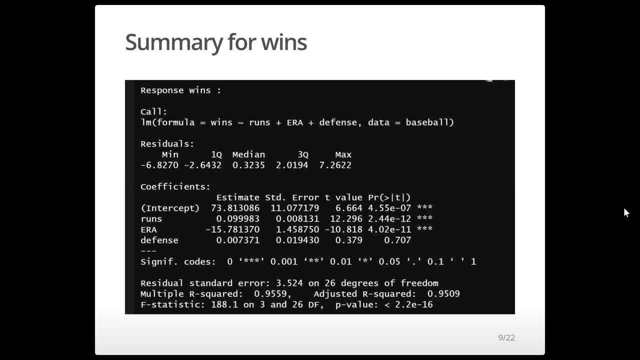 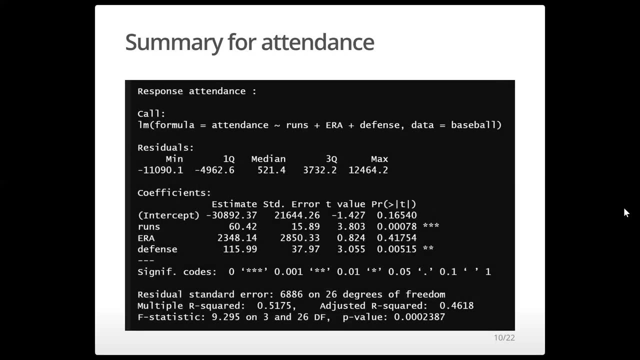 separate ln's. so it's going to give us the summary output for the regular model that we've already seen, with the outcome variable being wins, the response variable being wins, and then it's also going to give us a separate one for attendance. so here is the summary output. 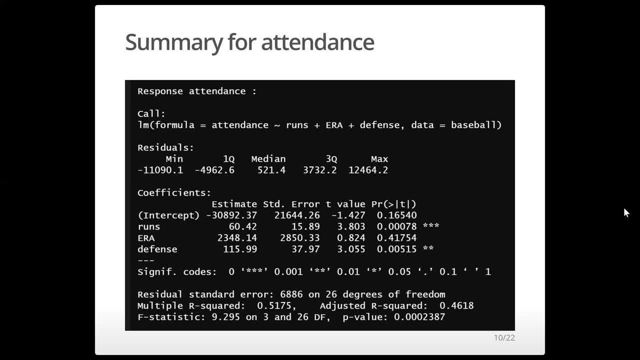 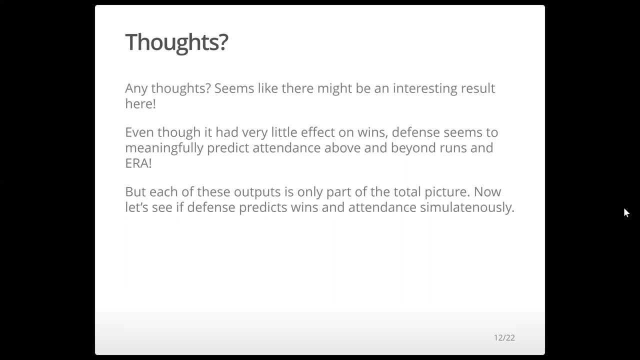 for attendance. so the summary output for the multivariate linear regression is just going to list both of these, so it's going to give us the separate linear regressions, and so do we notice anything sort of interesting about this result? so, even though it had very little effect on wins in our 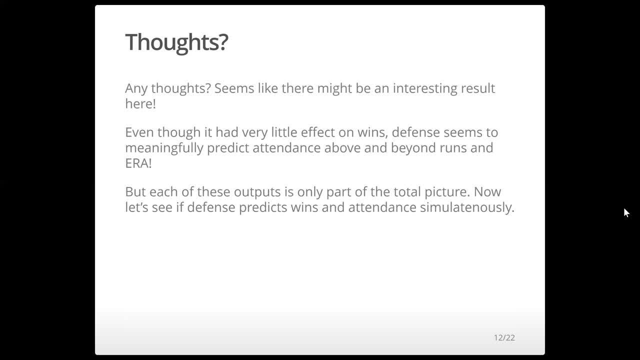 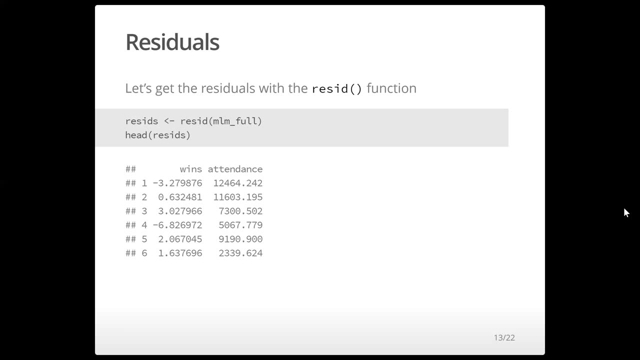 last slide, slide deck- defense seems to actually predict attendance above and beyond runs and era. but each of these outputs is just part of the picture. so now let's see if defense predicts wins and attendance simultaneously. so first we're going to get the residuals with the resid function, like we've seen. so 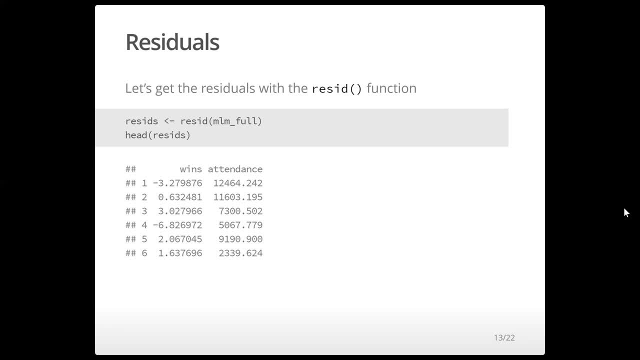 this is now two sets of residuals, so it's the residuals for wins and the residuals for attendance, from each separate multivariate or each separate multiple regression, and so i can transpose and multiply the residuals by themselves to get the sscp. and so this is from the full, the full model. so now i'm going to do the same. 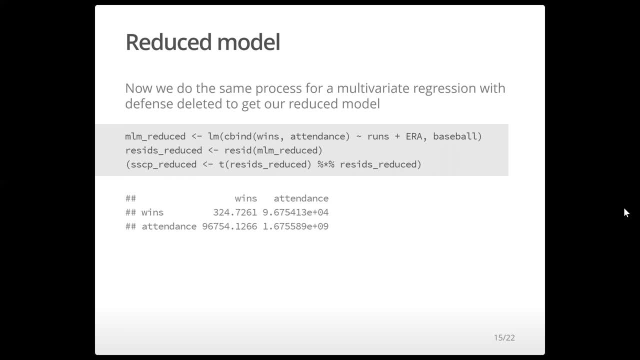 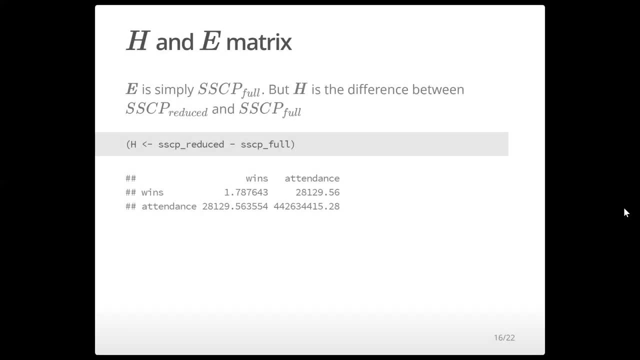 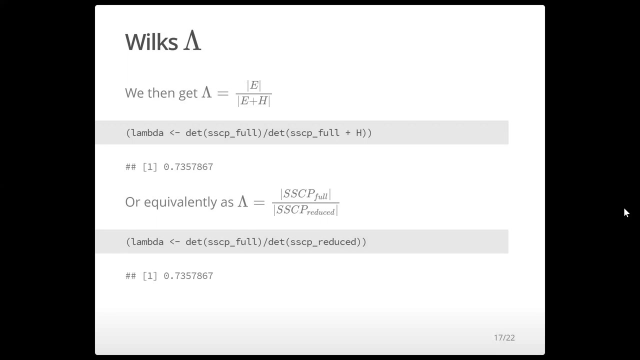 thing for a reduced model where i delete defense, and so now i get my sscp for the reduced model. and so what happened was we have two elements, for both is that we get lambda as the determinant of the determinant of e plus h. we simply divide the sscp. 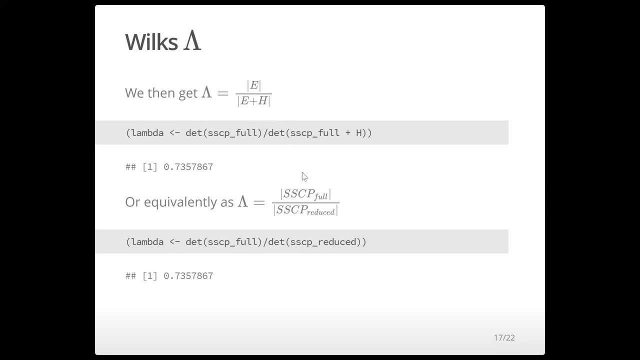 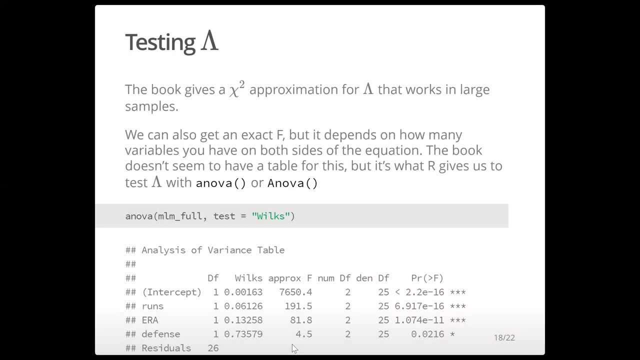 opposite, by theomma spends that 7p, which is making what we call save s. Dash by s with minus 0, that's output in R gives us the hypothesis matrix, here the H instead of the full and reduced. So it's good to know where these come from. 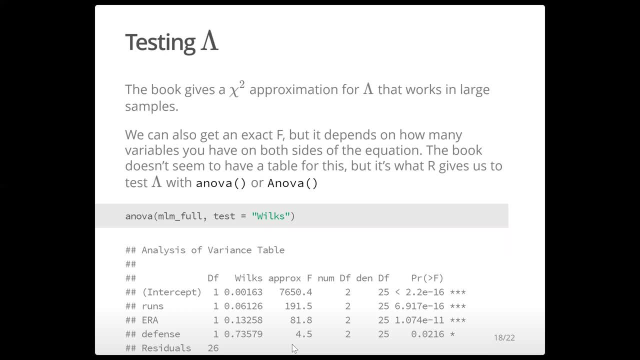 So the book provides a chi-square approximation for lambda that works in large samples, but we can also get an exact F. The confusing part about F, as we've seen in other cases, is that it depends on how many variables you have on both sides of the equation.